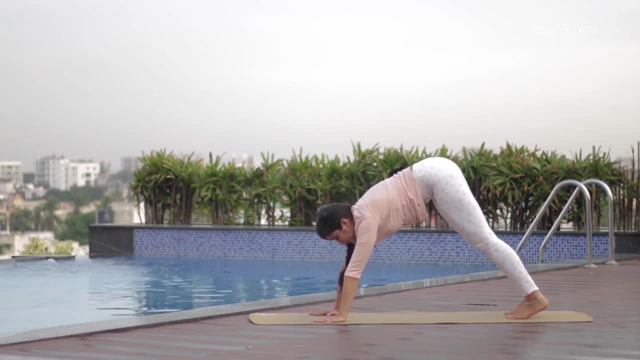 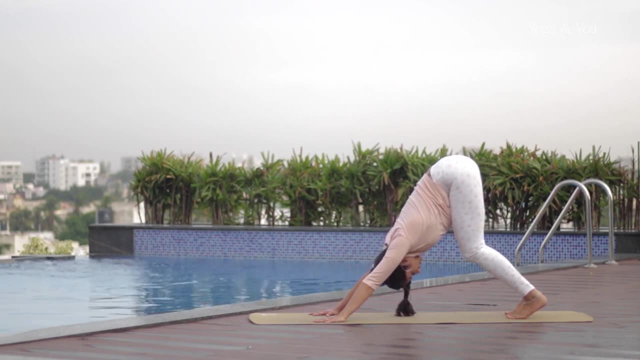 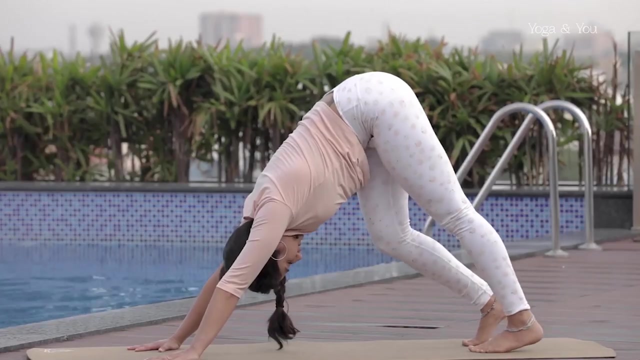 not really getting a good stretch here. Other than that, just push back with the hands and keep the knees bent. This is a much better position than that, So it'll really lengthen out the back. And now let's start walking out the dog. So bend one knee towards the chest, other knee towards the chest, Keep. 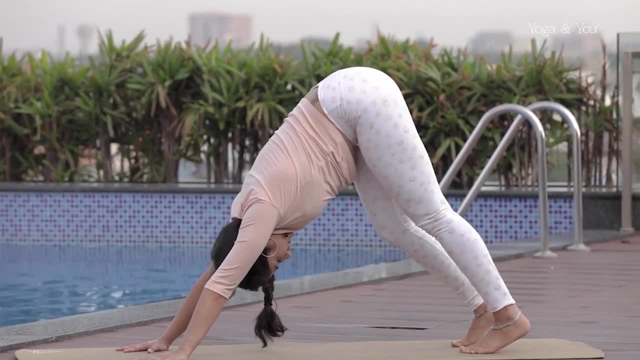 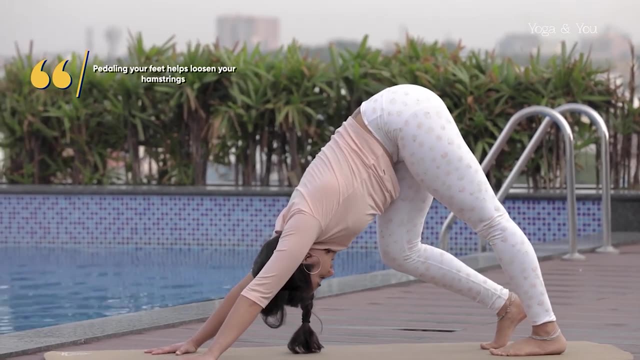 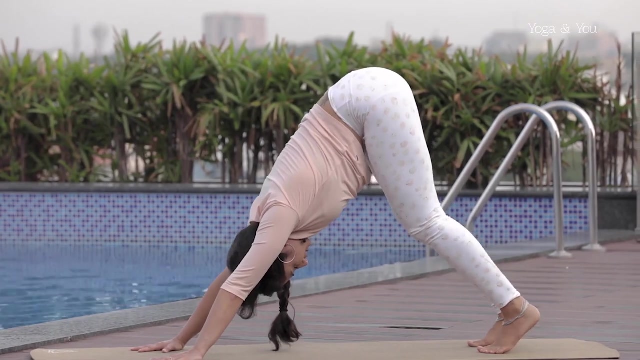 going One knee in other knee in For five: inhale one side, exhale other side. Four: inhale one side, exhale other side. Try to really slow down the breath. Breath should be the most important part of the practice. Two and one: 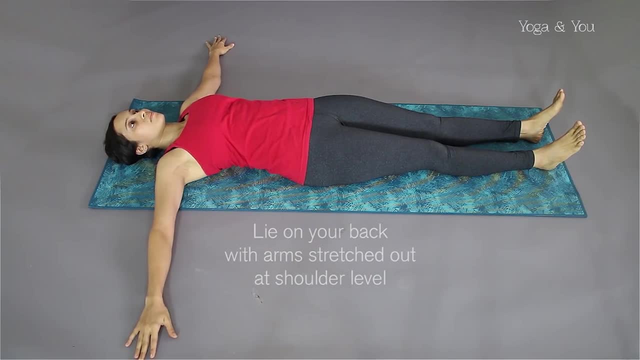 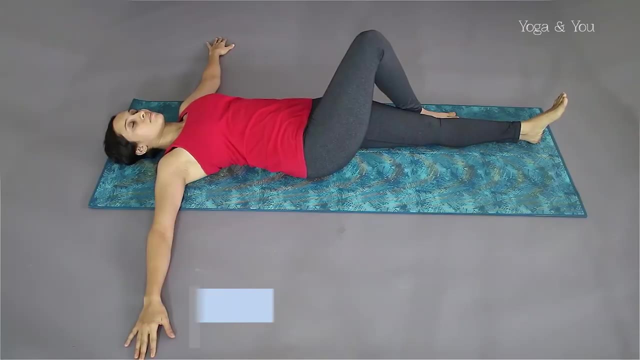 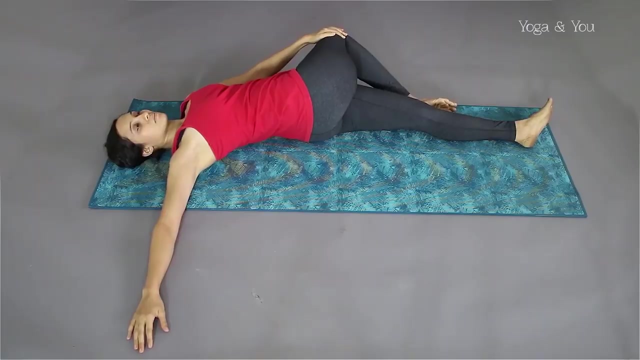 Lie on your back with arms stretched out at shoulder level. Bend right knee and cross it outside of your left leg close to the left knee. Slowly start twisting towards the left side. Use your left hand to put slight pressure on the bent knee. 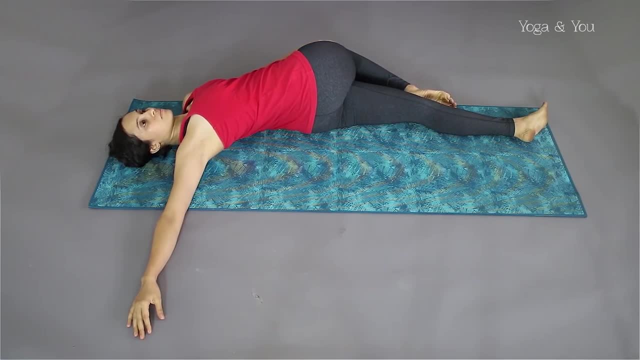 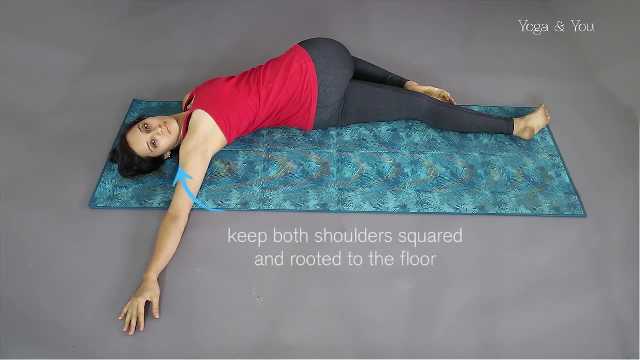 Push down towards the floor. If the knee is not touching the floor, it's still okay. Try to focus on your twist and stay comfortable. Try to keep both the shoulders squared and rooted to the floor. If the right shoulder is off the floor, it's no problem, Just try. 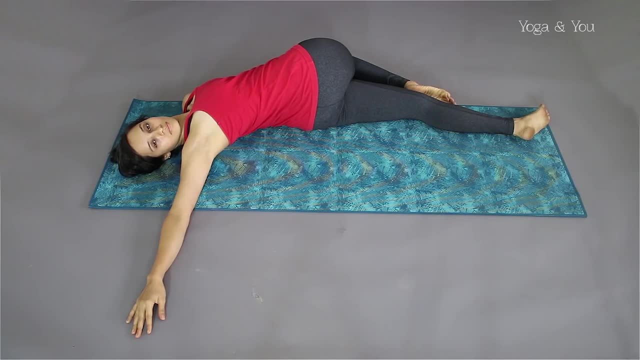 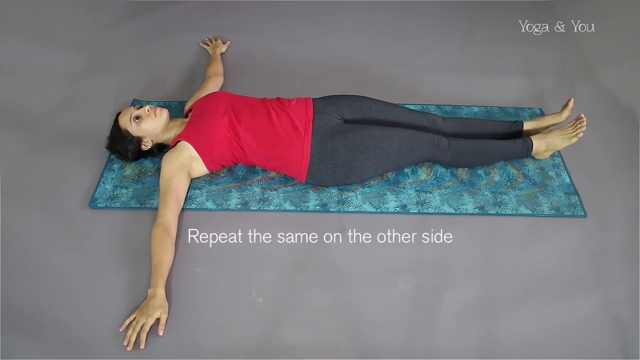 and be aware of it. Keep pressing it towards the floor and keep breathing into the twist. Stay on for 30 seconds or more. Slowly bring your knee back to stretch out your legs. Now we repeat the same on the other side. Bend your left knee to twist to the right side. 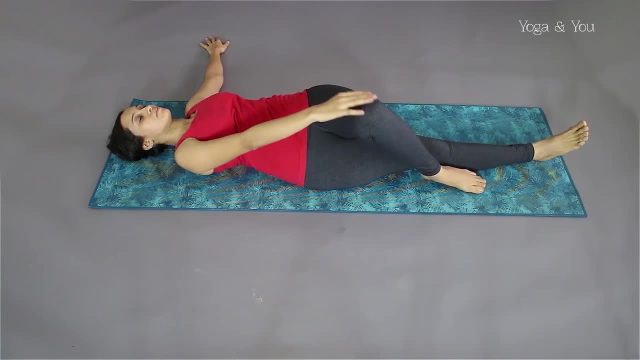 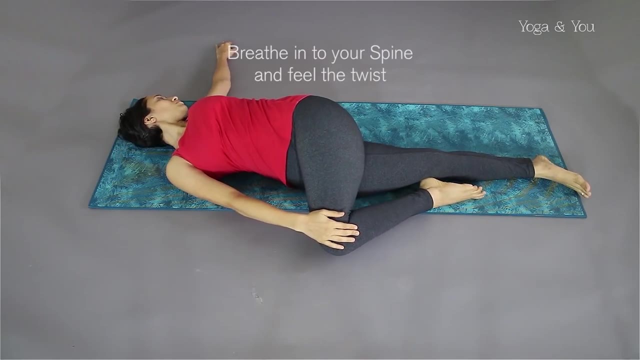 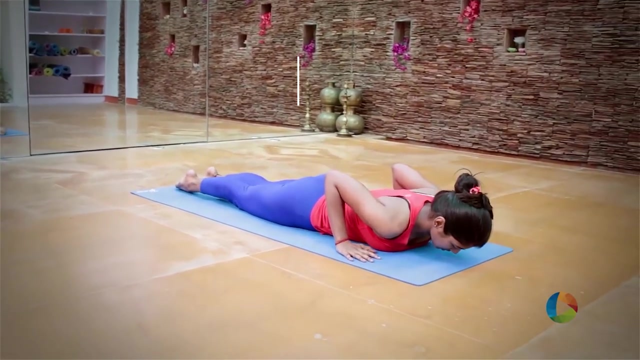 Use your right hand to press the knee down as much as you can. Press your left shoulder towards the floor, Breathe into your spine and feel the twist. So lie down on your abdomen. Try to keep your heel closer, your palms near your side of your chest. 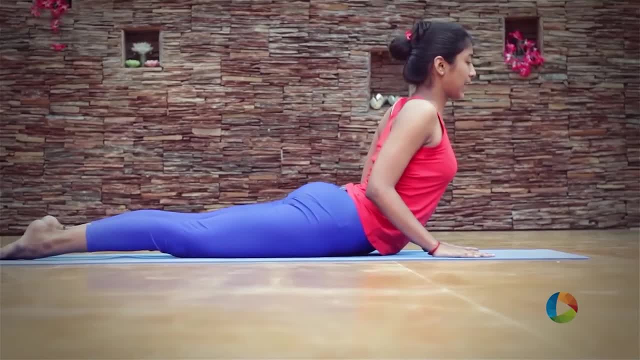 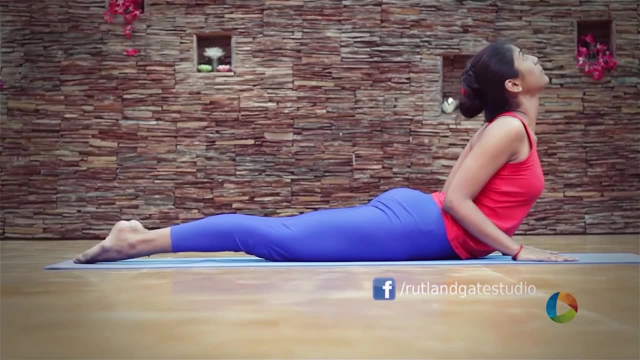 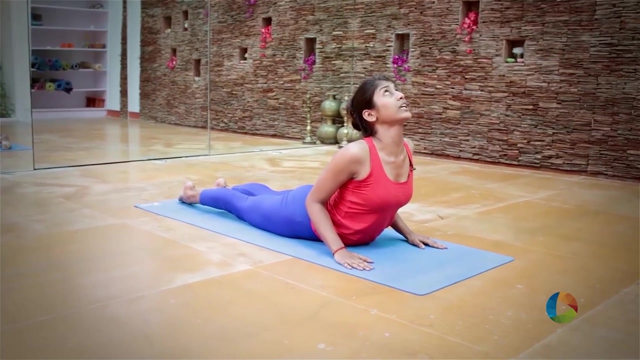 Now inhale and then come up such that the navel point touches on the mat Above your navel. nothing should be on the mat. Lift your chin up. look at the ceiling. Stay here for 5 breaths. When you stay here for 5 breaths, put all your upper body weight on your middle back. 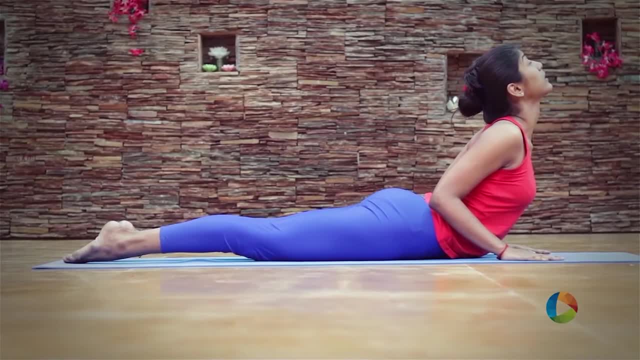 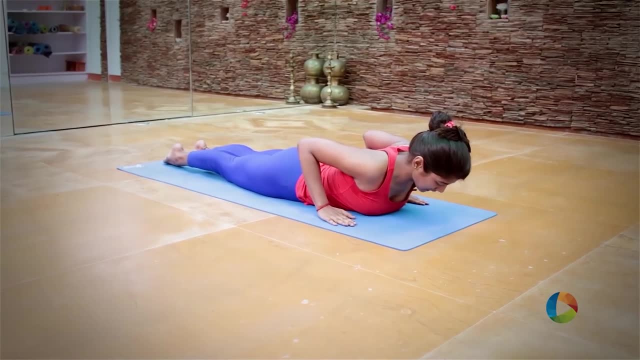 and strengthen your middle back as much as possible And exhale down. Now we will do one more variation in Bhujangasana. The same thing: inhale and come up such that the navel point touches the mat and gently lift your hands off the mat. 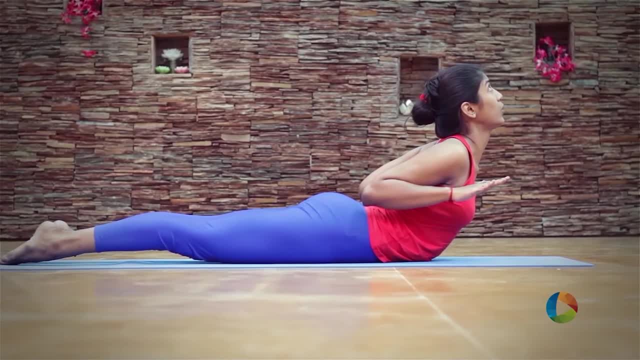 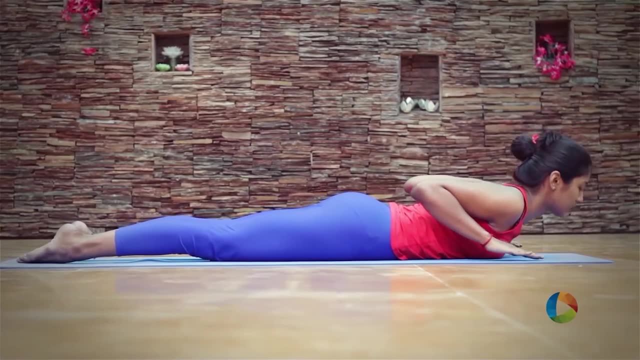 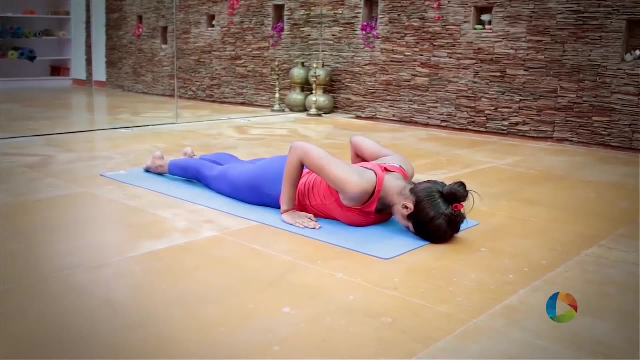 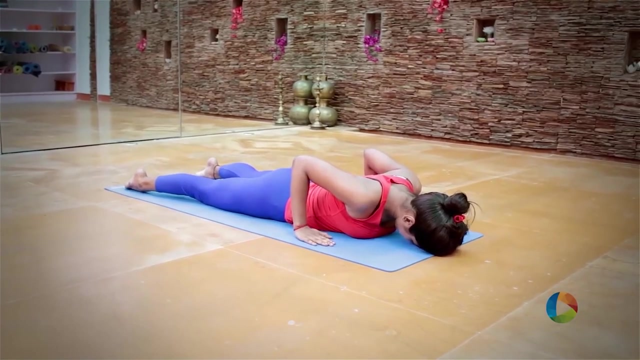 Stay here, shift all the body weight towards your lower back and strengthen your lower back. Exhale down. Now gently place your hands down in between your shoulders and your pelvic bone. Open your legs slightly out, Inhale and then come up. 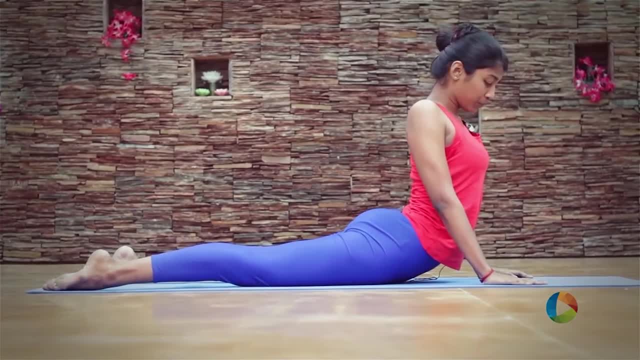 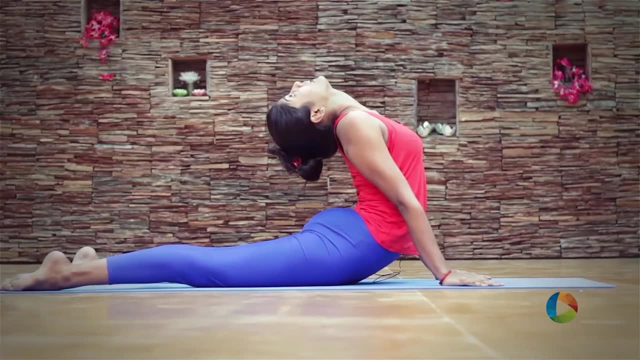 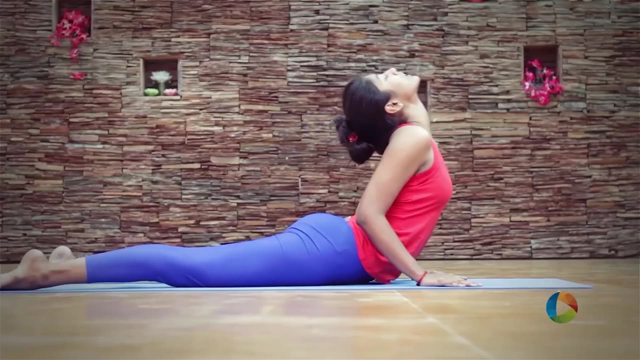 Now lift your navel above the ground level, Push your pelvic bone down. Procure your pelvic bone down and then elbow straight, Push the shoulders back, draw them back to the mat, Exhale down. Now the same thing again. join your legs together. 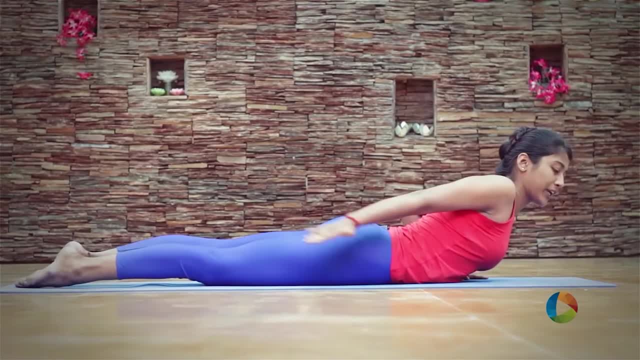 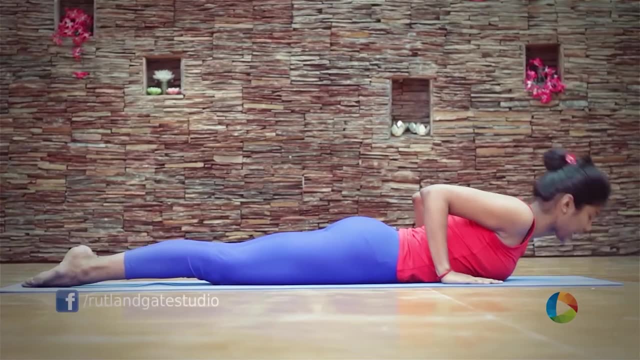 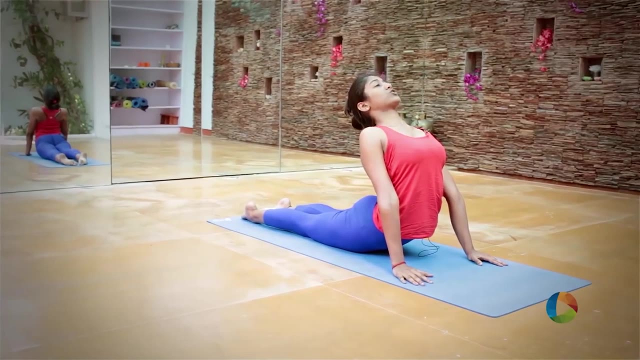 Heel together. When you join your legs together, your arch will not be more, but your spine stretch will be more. Inhale, lengthen your spine, Create a space between your pelvic and your ribcage And then arch back. 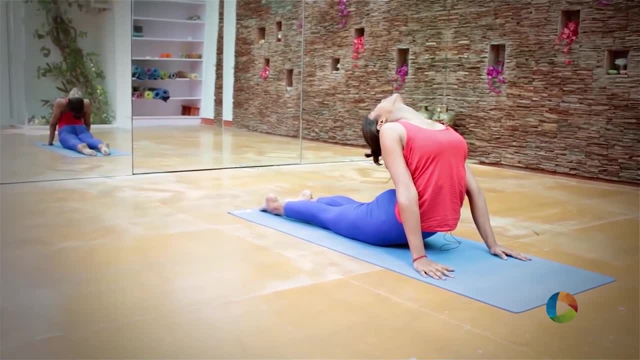 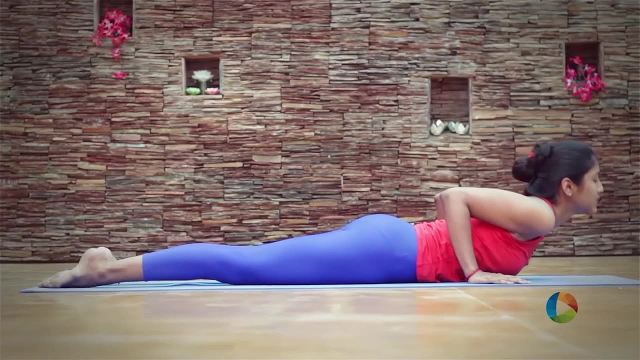 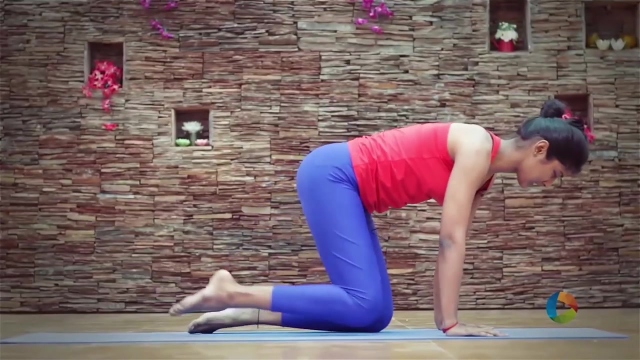 Squeeze your butt, drop your shoulders back and then arch Mouth closed. Upper jaw and lower jaw in contact with each other, Exhale down. Once you are done, you can go for Sushangasana. Stay here for two to three breaths. 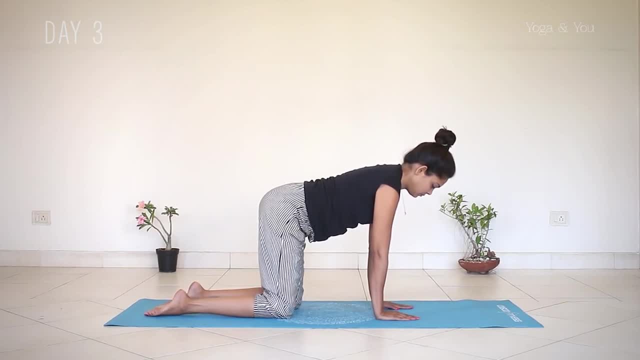 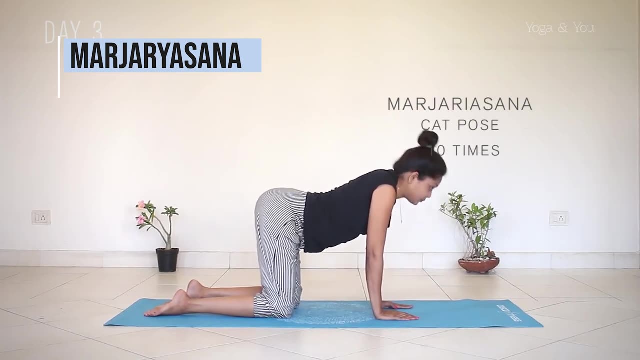 Now we are going to do the cat pose. Most of you know this Well. keep your arms and knees in the same line. You inhale, arch your back nicely, Chin to your chest and exhale. you look up to the ceiling and arch your back.